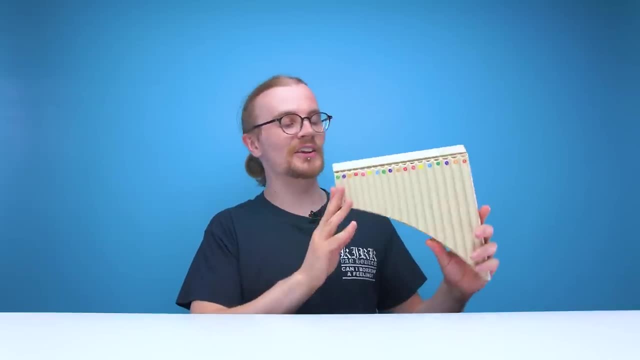 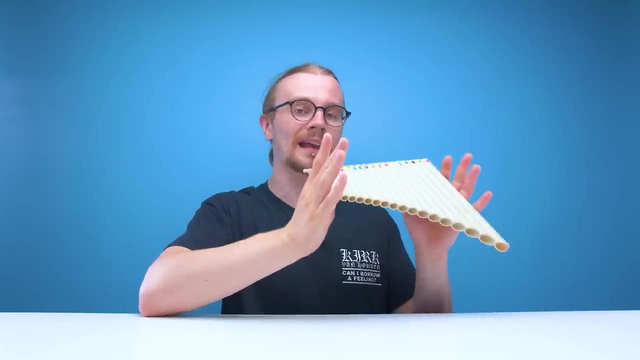 Now, there are loads of different types of pan pipes available online, but these ones particularly you can pick up for about £25 and they're really good. You get a very clean sound out of this one and it's very easy to pick up and play. You can even learn a few. 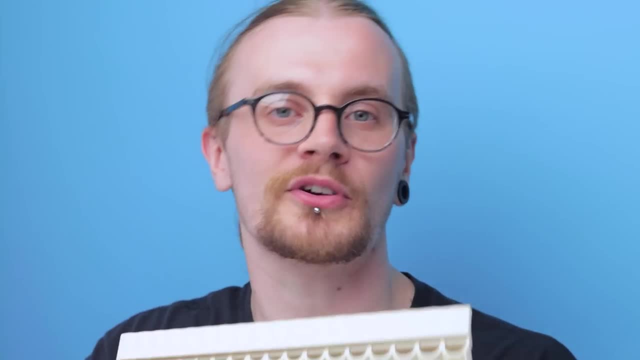 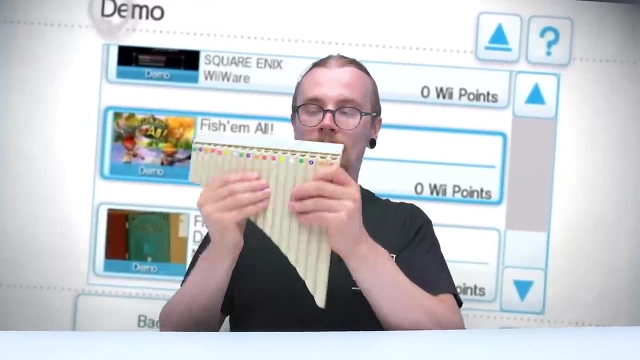 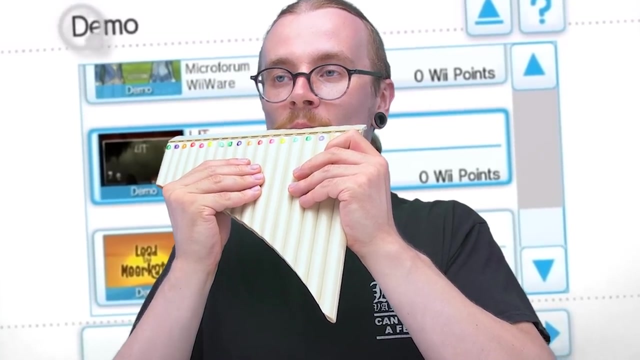 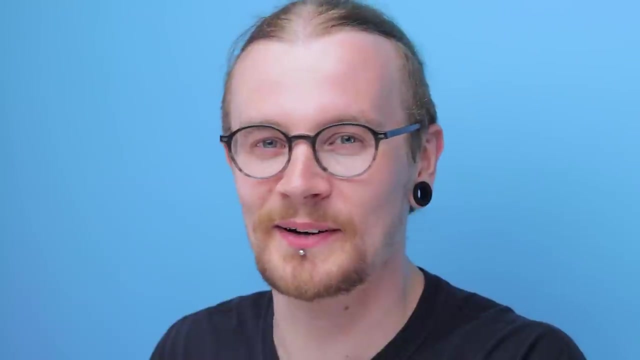 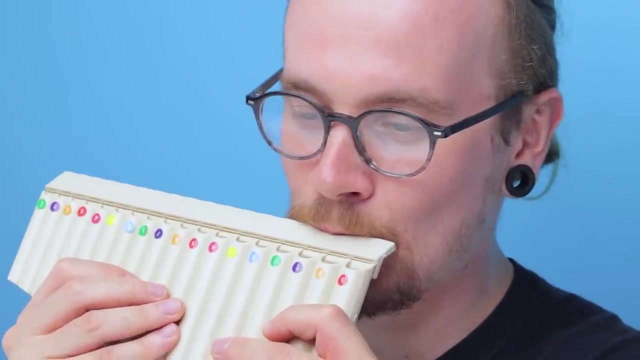 songs, or it's a very good instrument to freestyle on. And this is the part where I tried to freestyle on this one And it sounds absolutely awful, making my previous point completely redundant. I really screwed that one up. I have no idea what I'm doing. 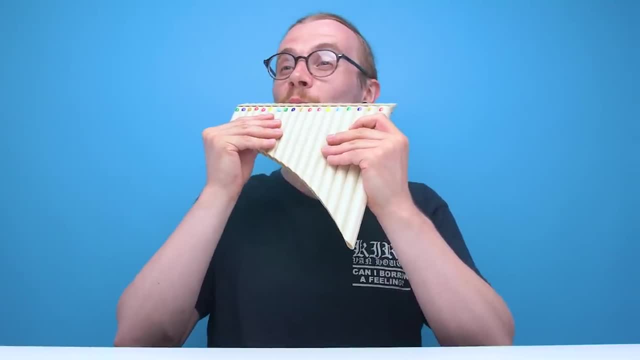 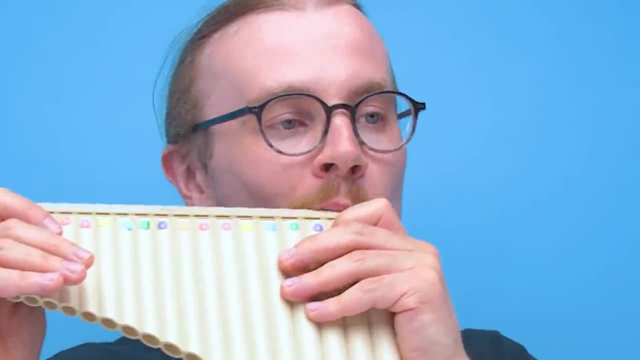 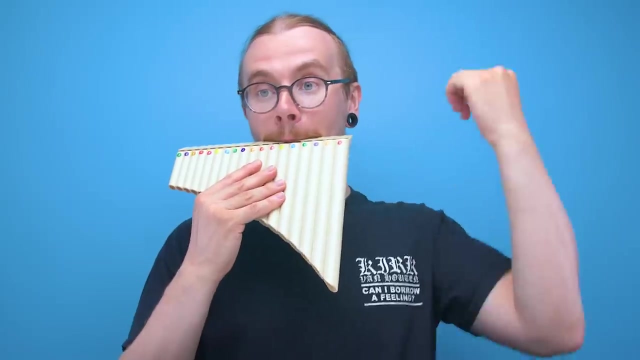 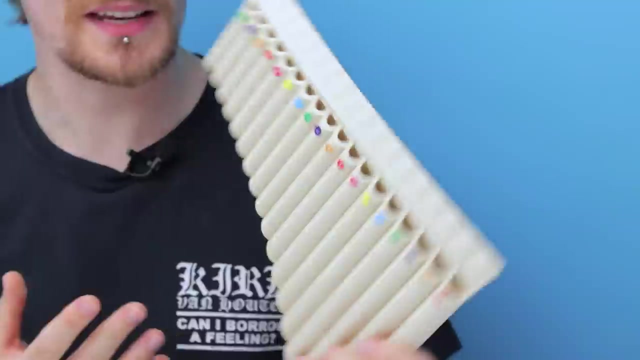 I think this pan pipe is a good one. for people who haven't played a pan pipe before, It's a great starting point. It's easy to pick up and play. It makes a good sound. What more do you want from a budget instrument? 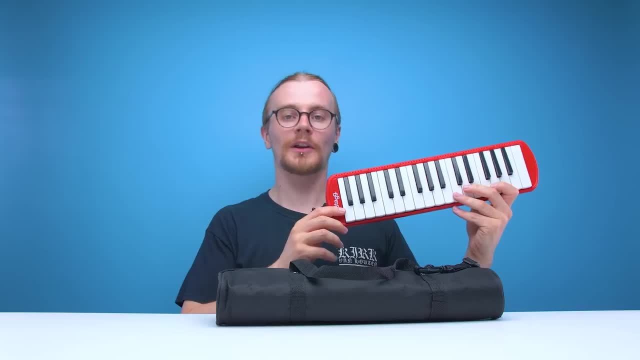 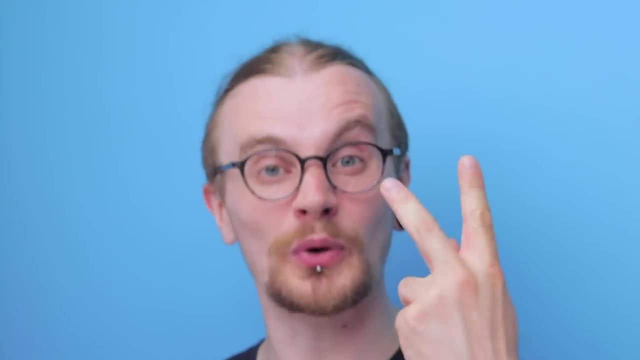 And at number 4 we have The Melodica. Again, It feels like a bit of a cop-out including this instrument in yet another list video, especially when you consider that we only have two list videos on this channel, including this video right here. 2 out of 2.. Well done. Now I'm going to assume that everybody watching 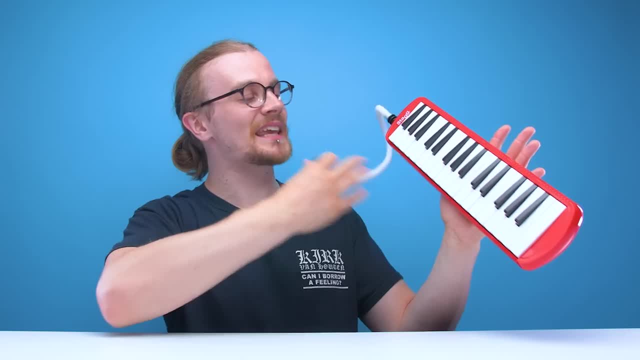 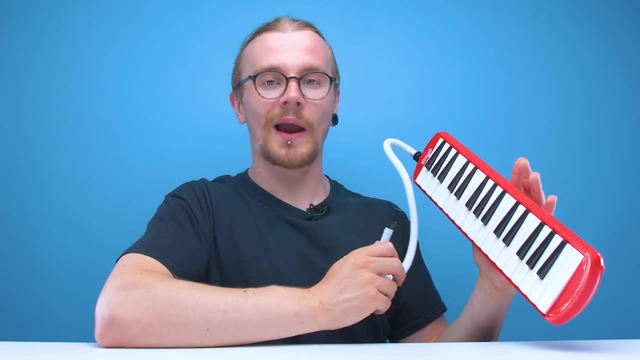 this video already knows what a melodica is, but, to keep it simple, it's basically a keyboard that you blow into. Simple as that And in true Looted style. despite having this instrument for so long, I still don't really know how to play it. I know I'm a terrible person. You don't need to tell me. 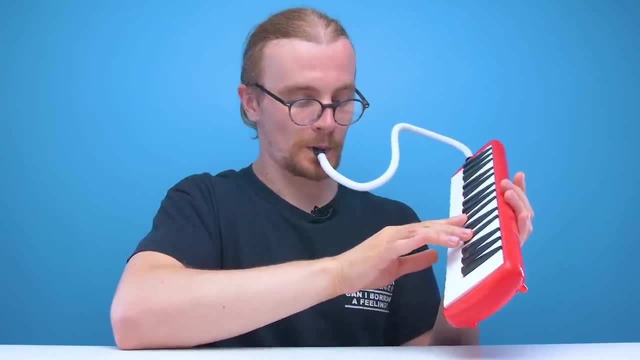 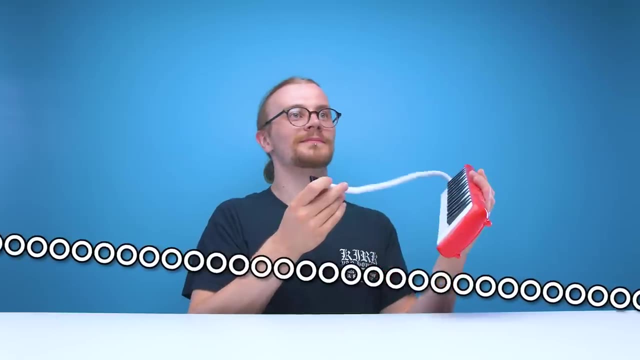 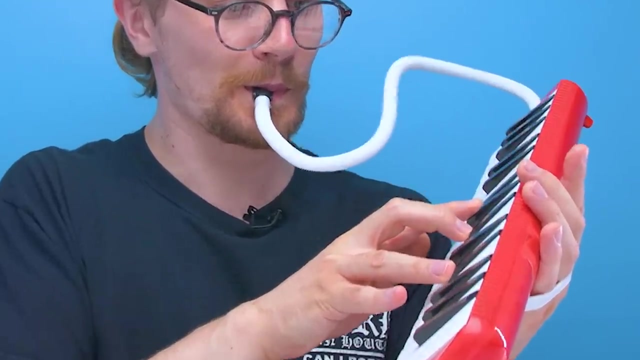 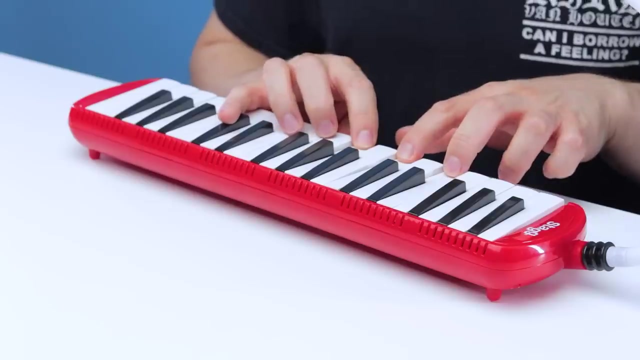 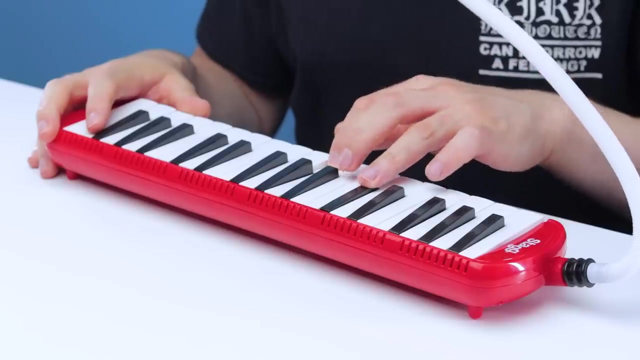 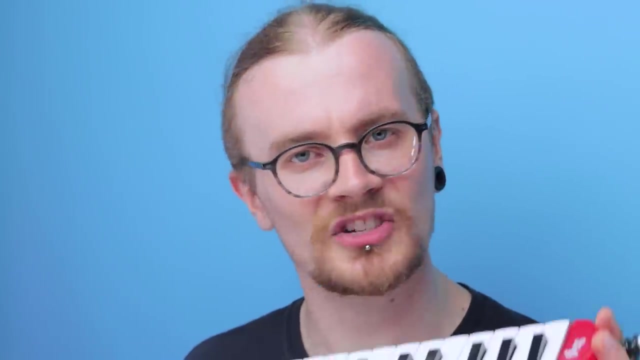 Nothing's changed. Noooo, Bye, I'll be back. Bye, Bye, Bye, Bye, Bye, Bye. This instrument sounds a lot more sinister than I remember, but maybe that says more about me than the instrument itself. I'm just a far shiftier bloke these days. 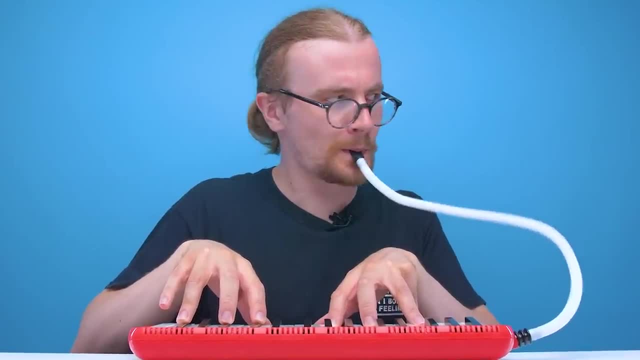 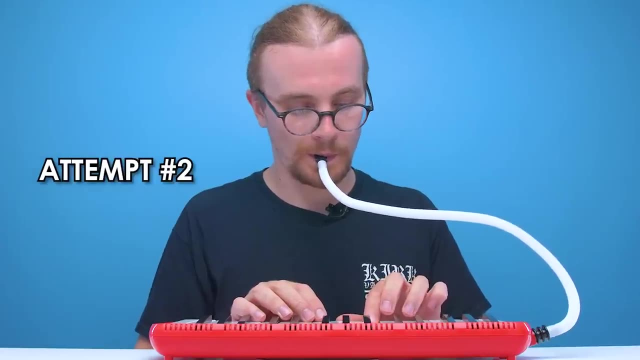 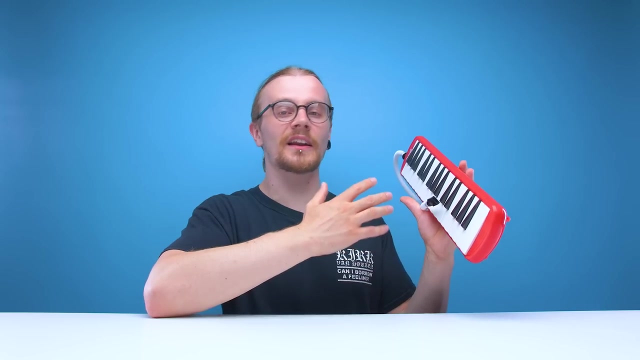 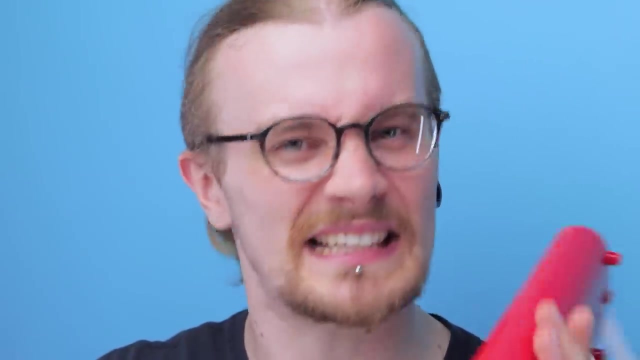 Or maybe that's just how melodic they sound after they've been left in the cupboard for like three years or so. It's once again another clean sounding and easy to learn instrument, despite me having never learnt how to play it, So I'm not a very good example, but take my word for it. 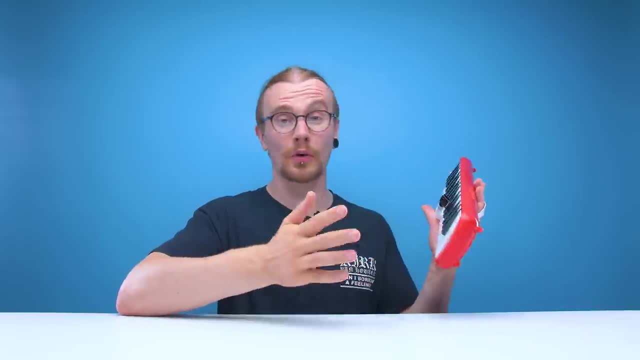 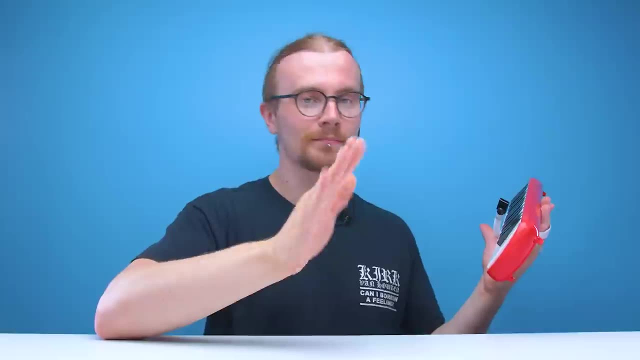 it's easy to learn And, of course, it's not like your regular electric keyboard which you need to power or anything. You can just take this anywhere and play it wherever, because you just need you and your lungs. Play it on top of a mountain, Play it under the sea. 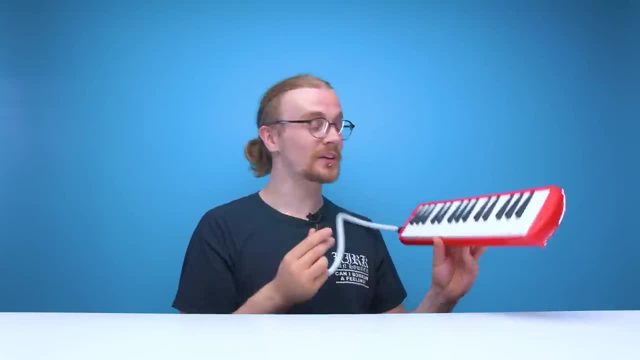 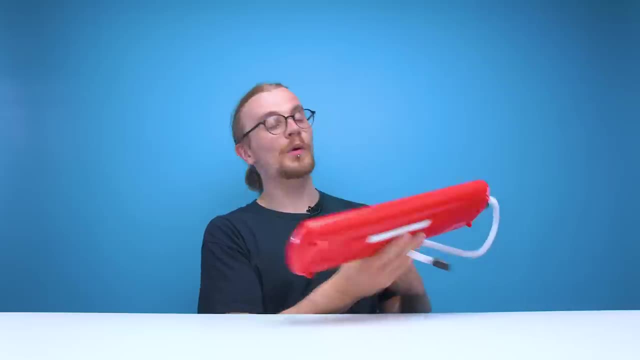 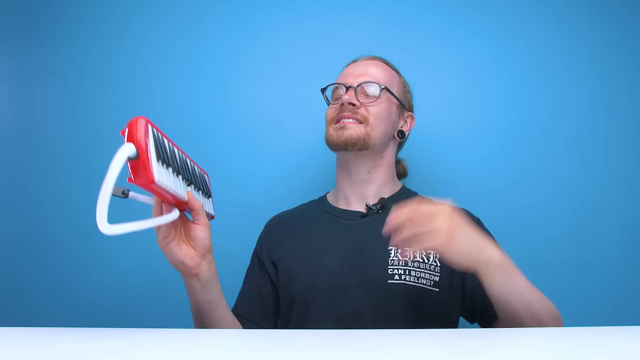 Maybe not that That might be quite hard. It's also a great two player instrument: One can blow, the other can play. And now, after talking about the Melodica once again on this channel, I think I can now confidently say that everybody who has subscribed to this channel is now sick of hearing about it. So 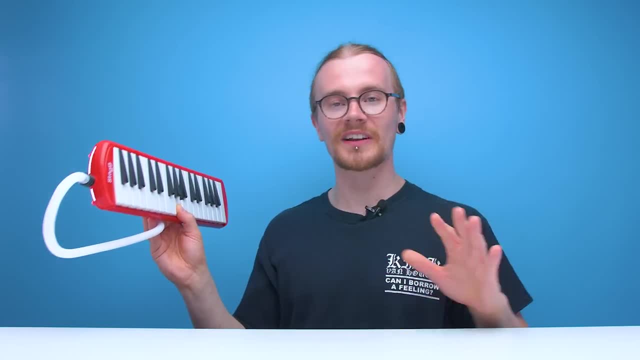 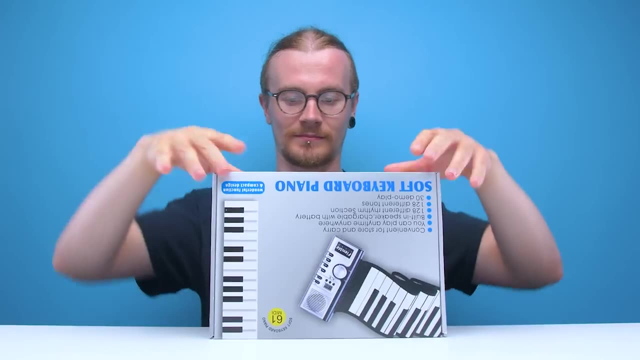 now I can retire it. It is good as gone. You're never going to see it again. Goodbye, Melodica. It was good knowing you. And speaking of keyboards, at number three we've got The Rollout PE. 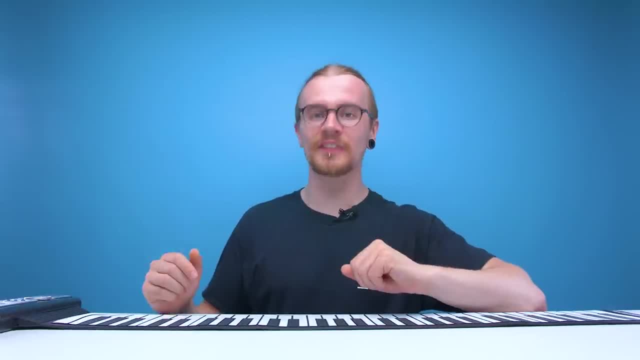 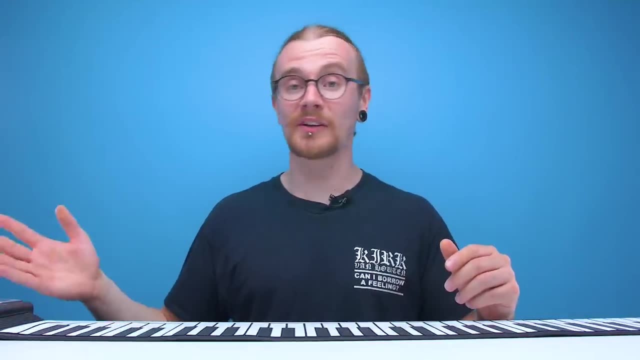 Now, I know we didn't really praise this instrument when we originally did a video on it, but it is a very versatile piece of kit For one. you can take it and play it pretty much anywhere. It's battery powered or you can power it via DC, And it also has 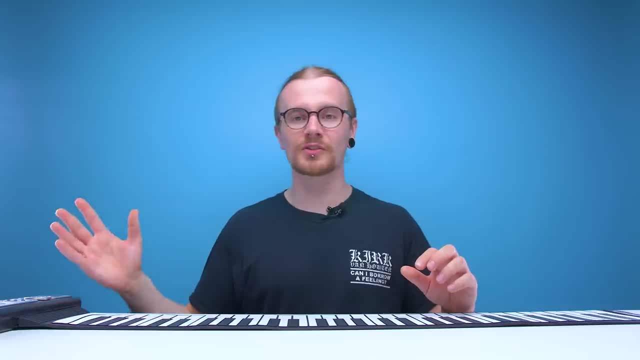 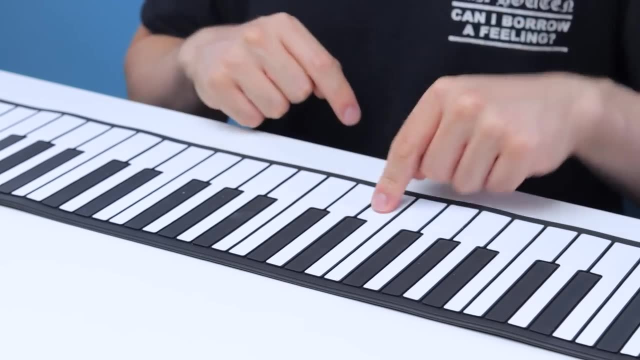 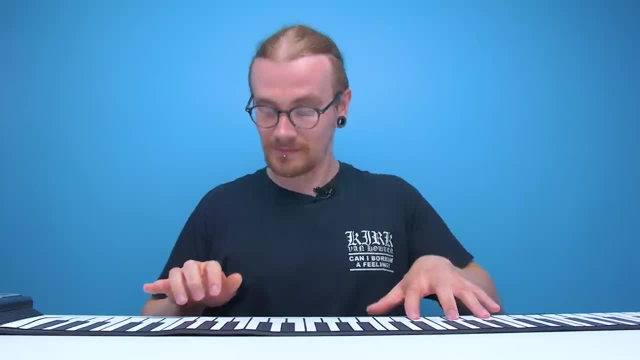 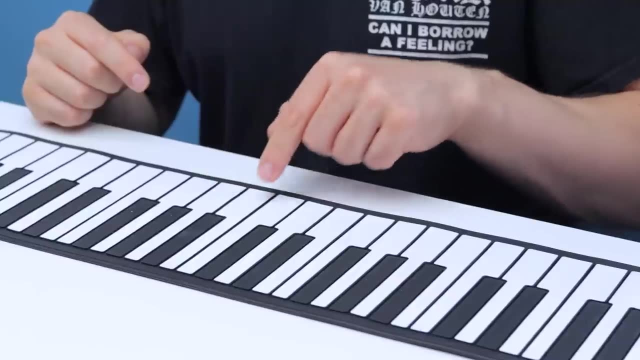 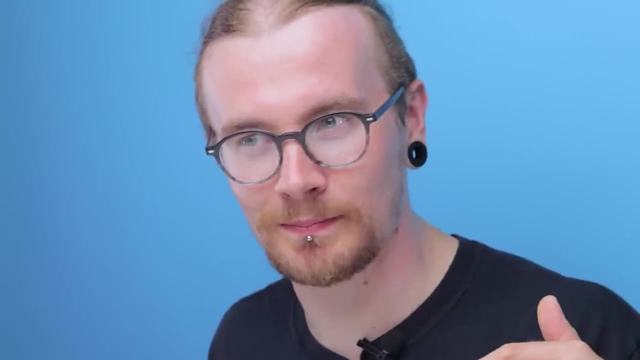 I don't know, And you can even get some weird sound effects out of this thing, Not actually sure what that sound is: Scratching of a deck or really bad birds. Your guess is as good as mine. Ah, that's birds, Or is it a car alarm? 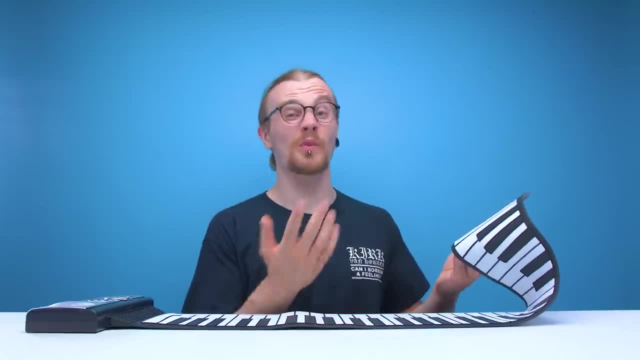 Now, of course, this thing isn't going to be as good as a top quality keyboard. I mean for one, not a great keyboard, But for the other. there's some things that you want to keep away from, like the so 온 is pizza App vị tengок a bộént н tapes c? 그래서. 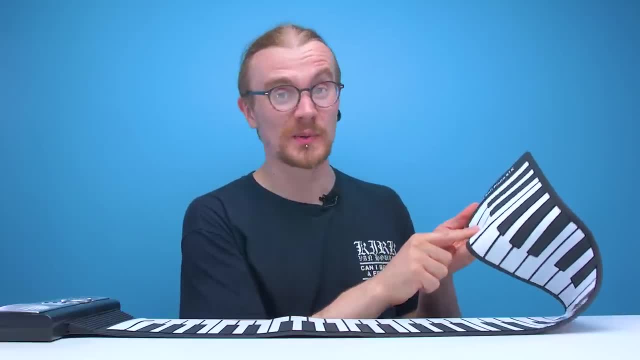 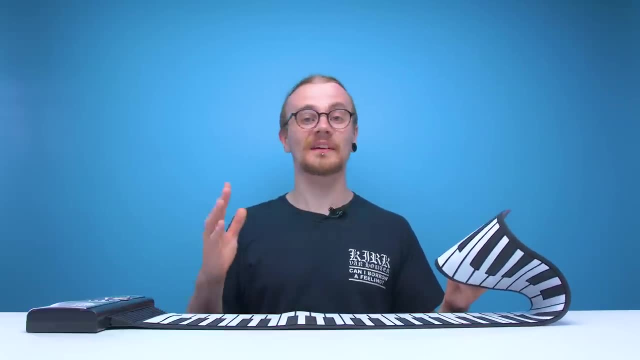 The keys really aren't all that great. They're made of silicon, which means they're squidgy, They don't give much feedback. But that doesn't take away from how versatile this keyboard piano is, and I think if you're looking for a more Compact and movable keyboard, This is a good place to start. 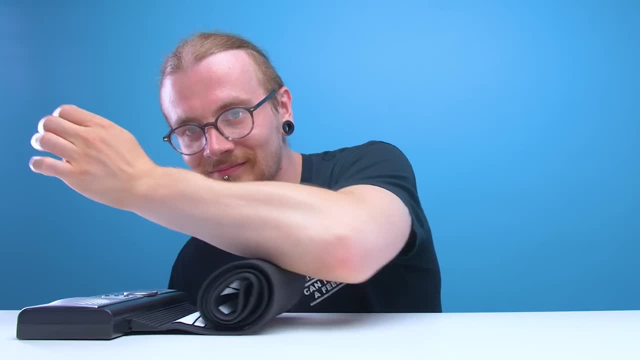 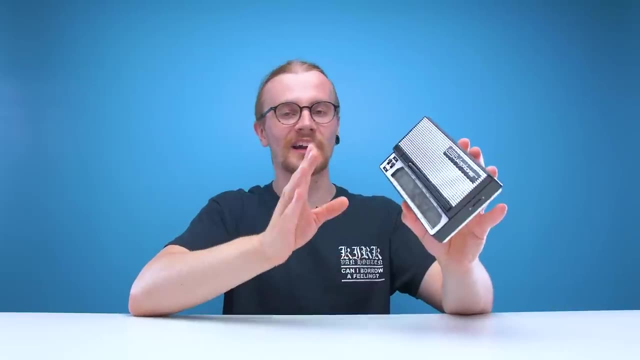 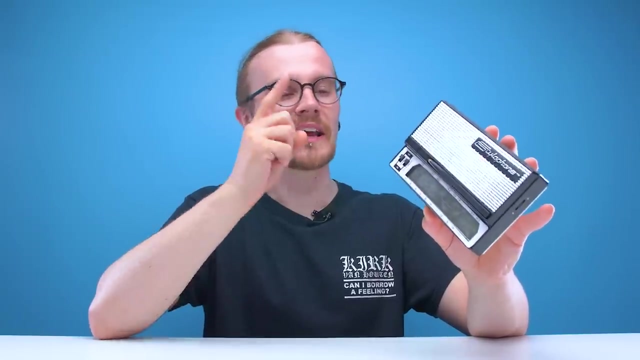 And at number four, we've got the Original stylophone. now, if you want the full stylophone experience, I would suggest that you check out the gen x1, but that is significantly more expensive than the original. So this time around, this little guy gets our pick. now. 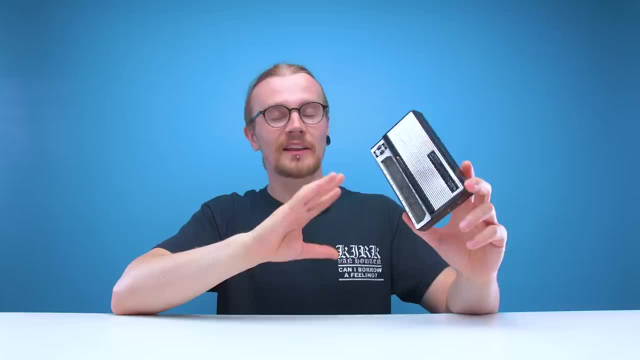 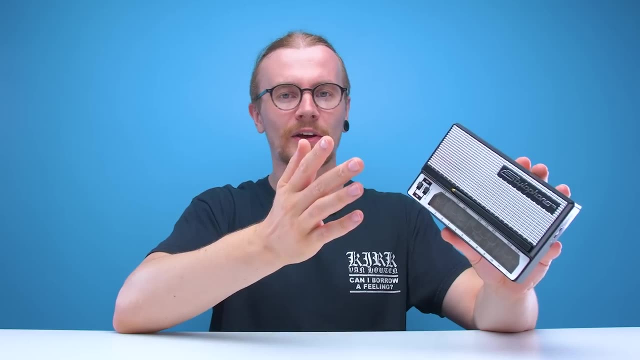 I think I can safely say that this is one of the most famous pocket synthesizers out there. This thing is turned up in music by david bowie, a load of other artists from around that time period, and it just has a Very unique and retro sound to it. Now, I don't know where they got the idea of this thing being a pocket synthesizer. 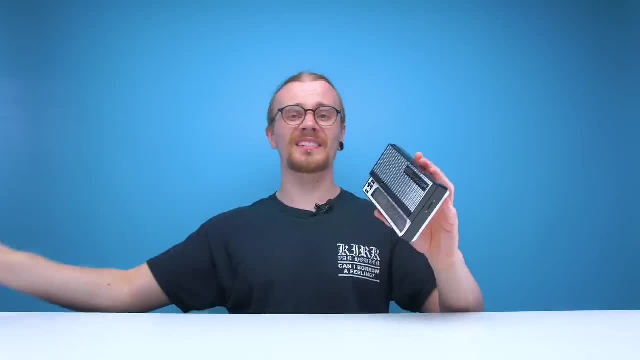 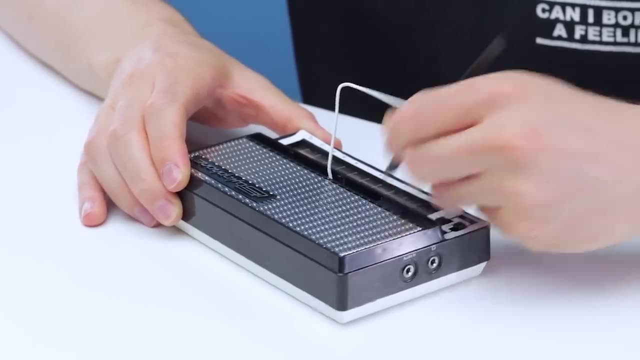 I mean it says it on the box- the original pocket synthesizer. But let's be honest, unless you're a goth kid from the early 2000s, This thing ain't going in nobody's pockets. It's fun, It has A very basic electronic sound and it's very open for customization. 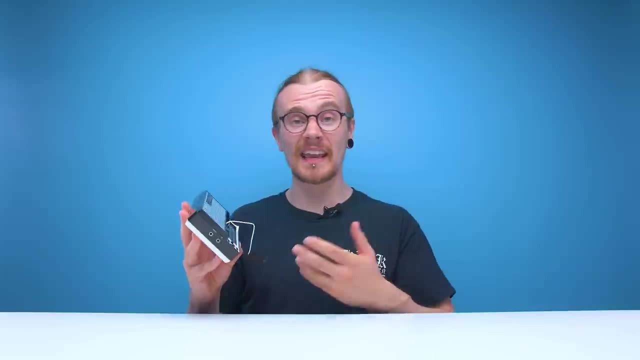 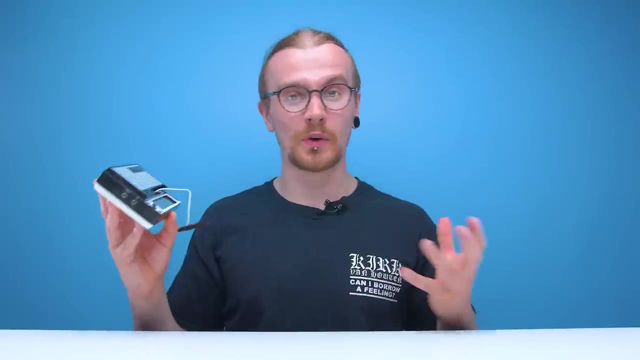 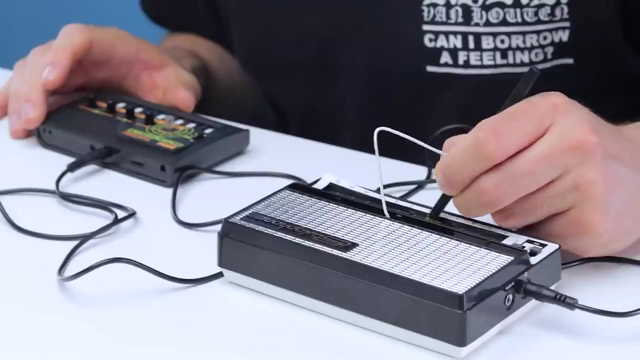 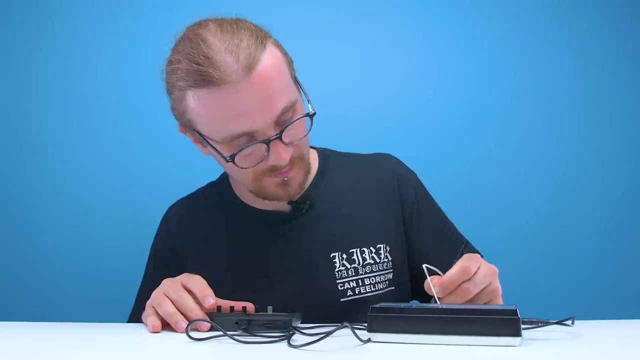 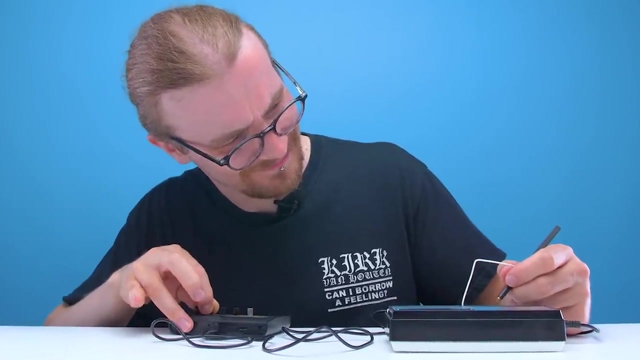 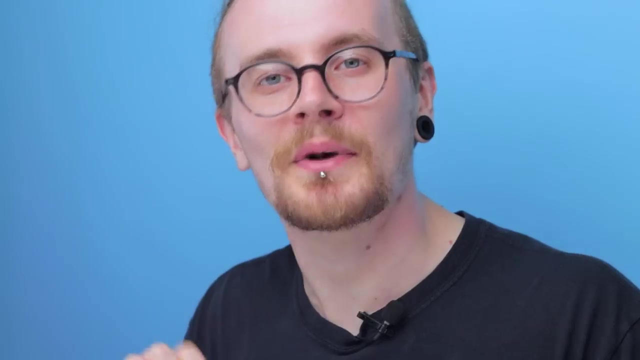 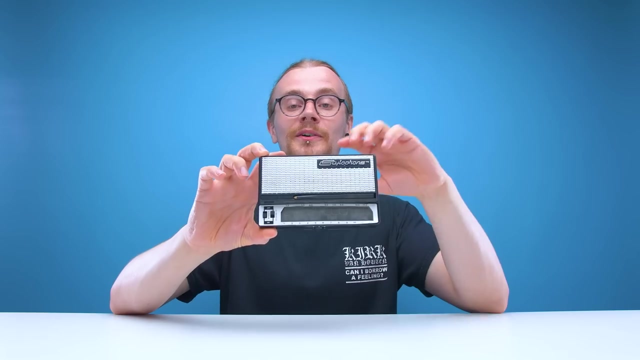 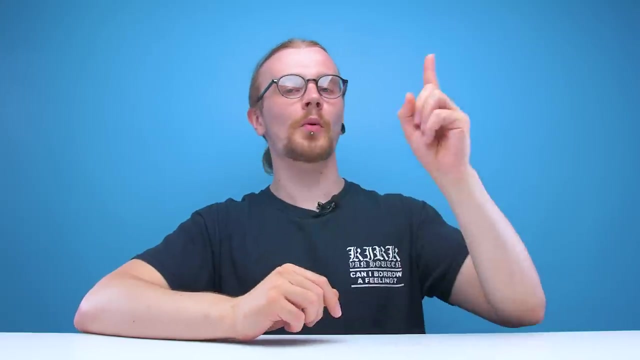 Of course, unlike the gen x1, you don't have many options when it comes to adding delay and all sorts. But you can plug this into pedals. You can plug this into different synthesizers and just make some weird and wonderful sounds with it. example. It's a great little electronic instrument. if you're looking for something with more of a retro sound and retro look, you can't go too wrong with the stylophone. and then, of course, there's other versions of the stylophone which you can then upgrade to. so you've got options. and before we get to number one, let's go through some honorable mentions. 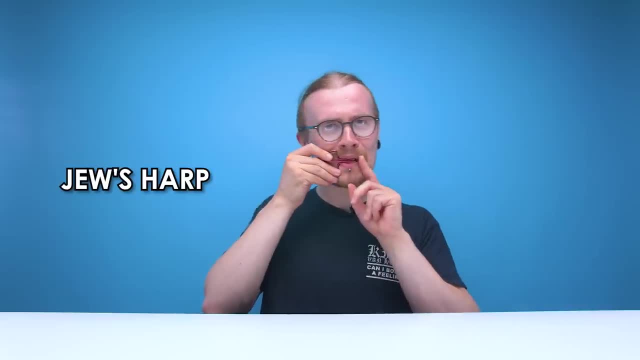 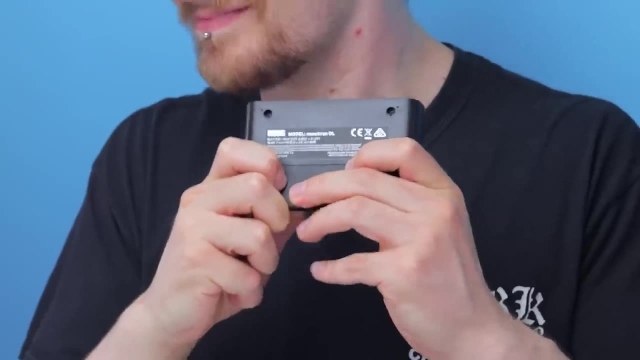 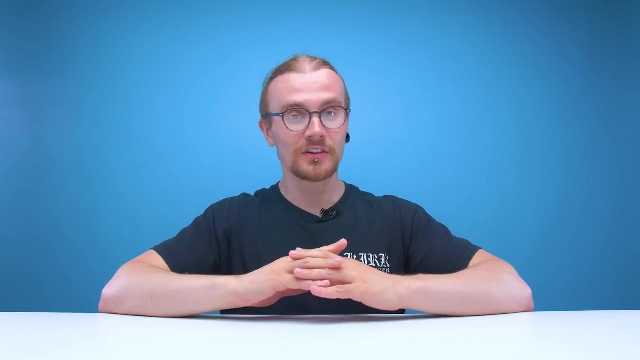 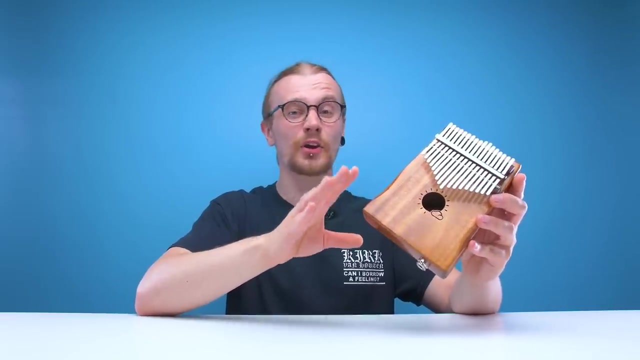 ow, And finally, at number one, our favorite budget instrument that we have ever tried on the channel. it is The kalimba. Unfortunately, we don't have the original kalimba, which we checked out on the channel like three years ago because they were cheaper.